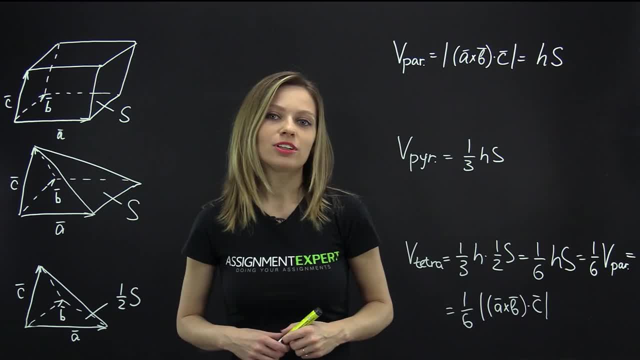 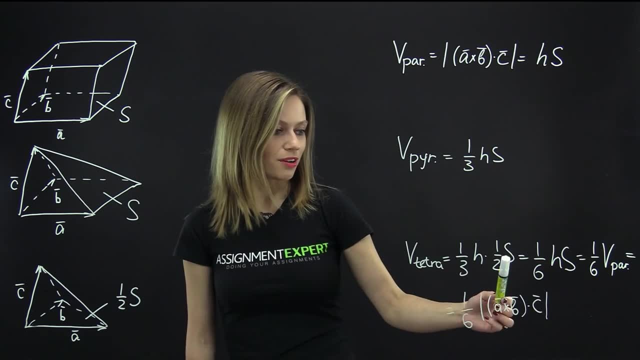 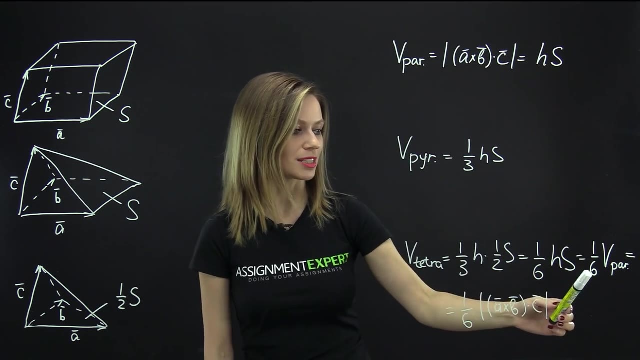 area of a corresponding parallelogram. So its volume is calculated as follows: One third times H times one half of S. We have one sixth times HS, and HS is equal to the volume of a parallelepiped. So we have one sixth times volume of the parallelepiped, or we can substitute our. 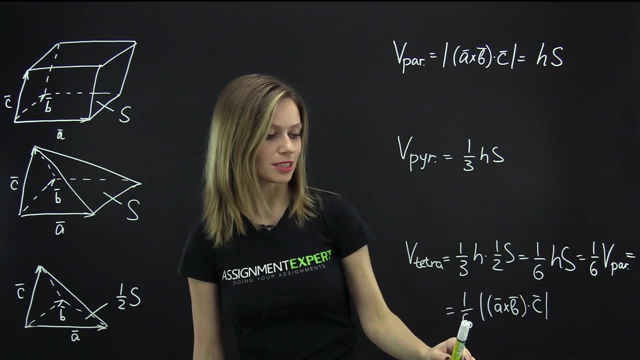 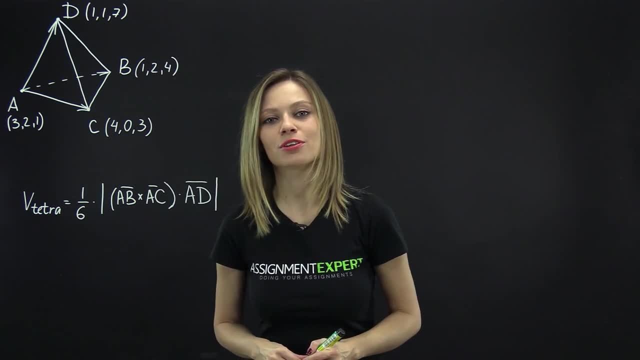 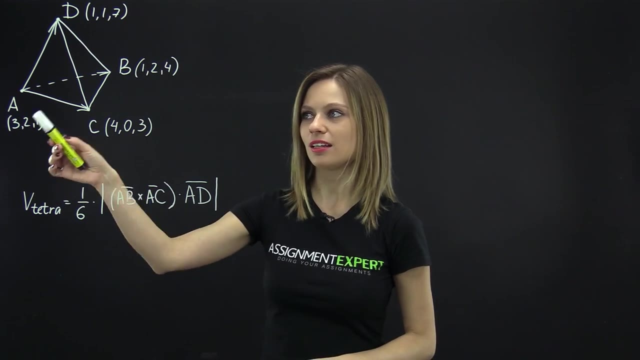 formula for the scalar triple product. and we have one sixth times the absolute value of A, cross, B, dot C. As we remember, the vertices of our tetrahedron are the points A, B, C and D, So we can say that it is built on the vectors A, C, A, B and A, D. Thus its volume is calculated as one sixth. 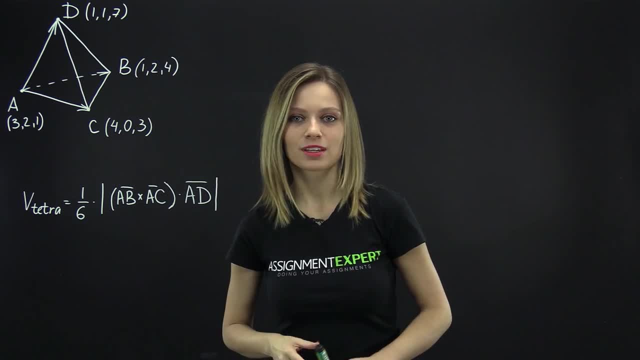 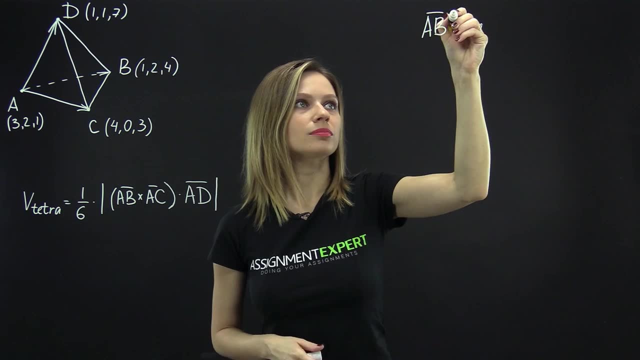 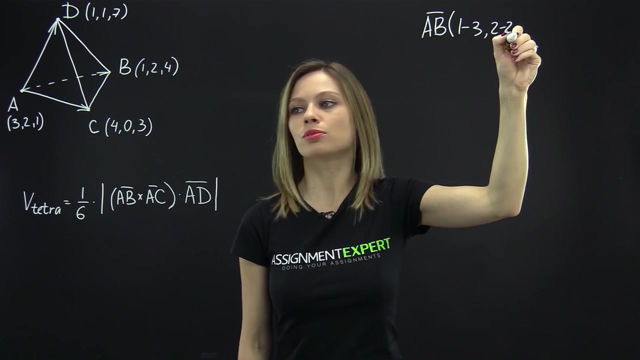 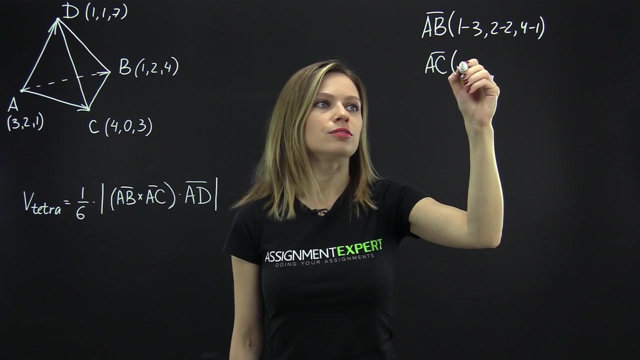 times the absolute value of the scalar triple product of these vectors. So let's find the coordinates of these vectors. We have that A. B has coordinates one minus three comma. two minus two, comma. four minus one. A C has coordinates four minus three, zero minus two, three. 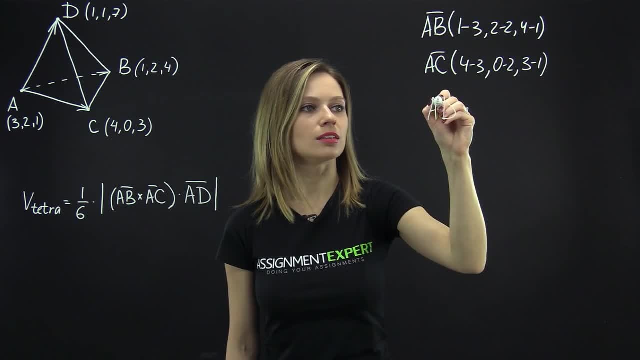 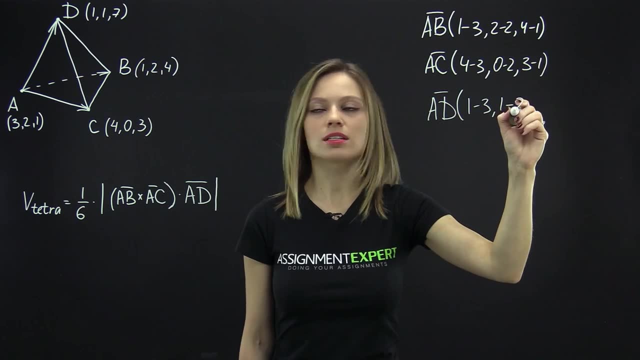 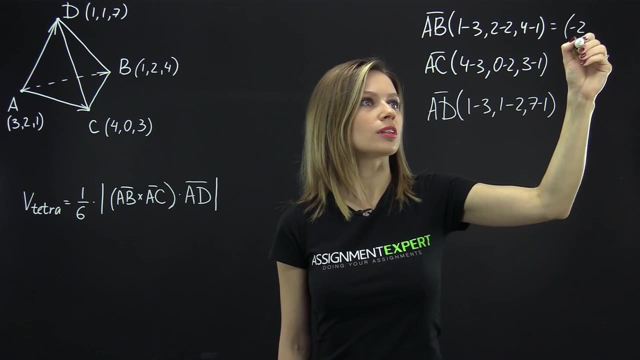 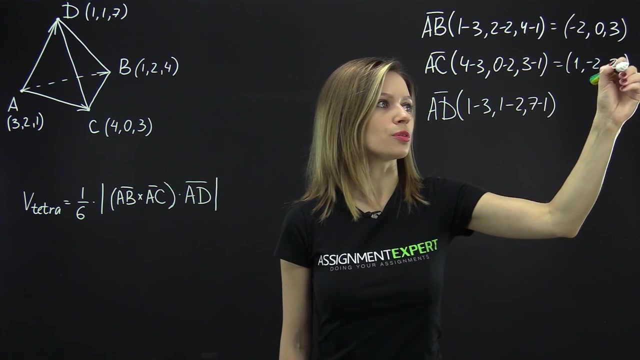 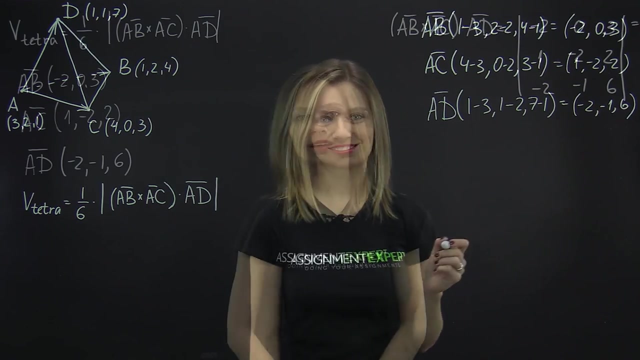 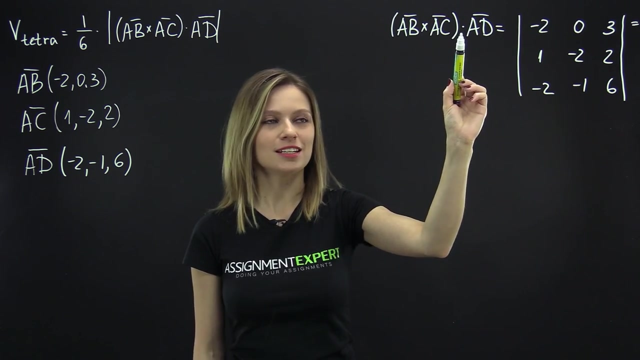 minus one and A D has coordinates one minus three, one minus two and seven minus one. So if we calculate that we'll have negative two comma zero comma three, one comma negative two comma two and negative two comma negative one comma six, Let's calculate the scalar triple product of the vectors separately. So A B cross A C, dot A D is. 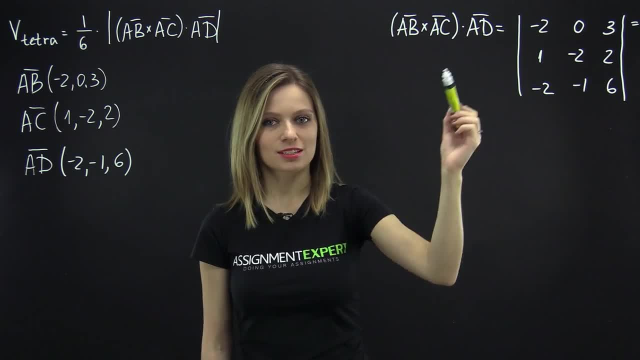 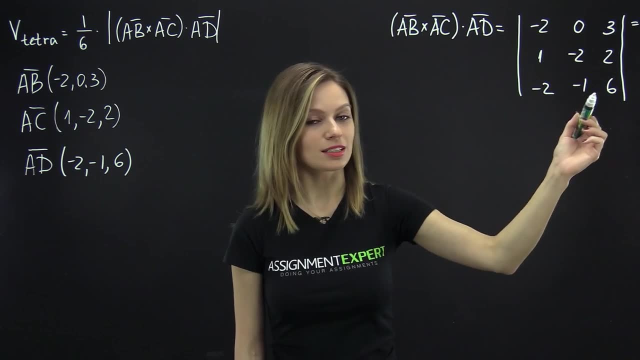 equal to a determinant of the matrix of the coordinates of these vectors. So we have determinant of nice: two comma zero comma three comma one comma two comma two comma one dash three comma two slight ****. We'll solve it using the primers rule, So we go like this: 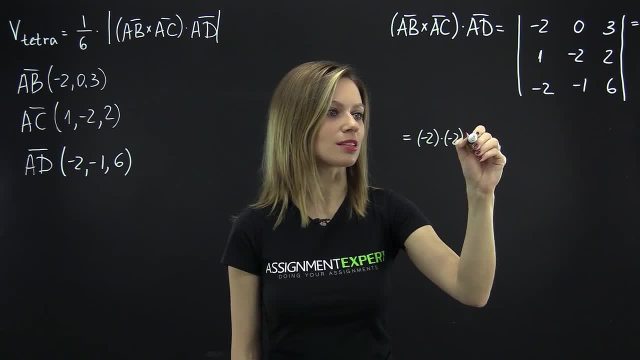 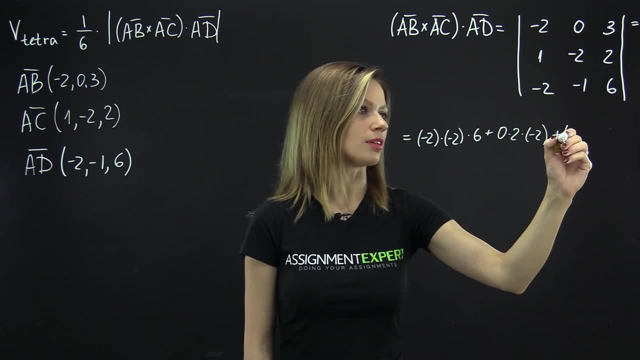 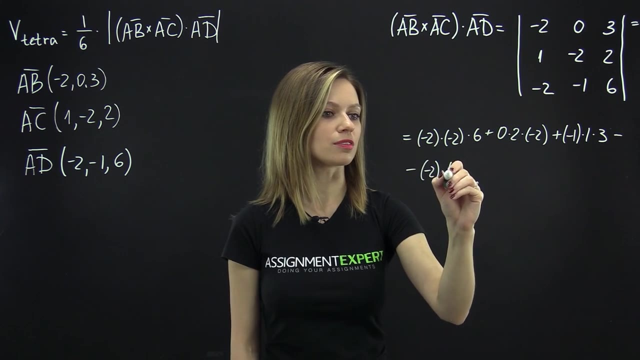 negative two square root of zero comma two plus negative two. two plus six plus zero plus one comma times two squared minus two, four comma two comma four minus three comma two, not just two comma negative two comma negative two comma negative two我们 statements here. Then we have read è: